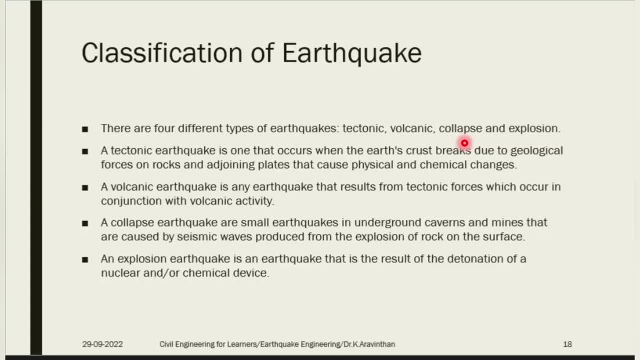 How the minerals are being mined is by detonating. So you have to explore the rocks. Explore the rocks below the earth or the surface. When you want to make tunnel, you are going to explode. The adjacent soil gets disturbed and it makes a small vibration and the waves are getting generated. 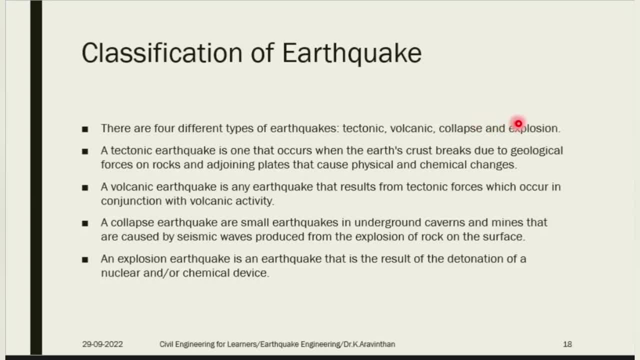 This is much smaller than volcanic earthquake. Last type is Explosion. Explosion is due to manmade. The earthquakes are natural, made, That is. tectonic earthquake is natural. Volcanic earthquake is also natural, But this collapse and explosion. If you are making tunneling, then that is a collapsible mode. 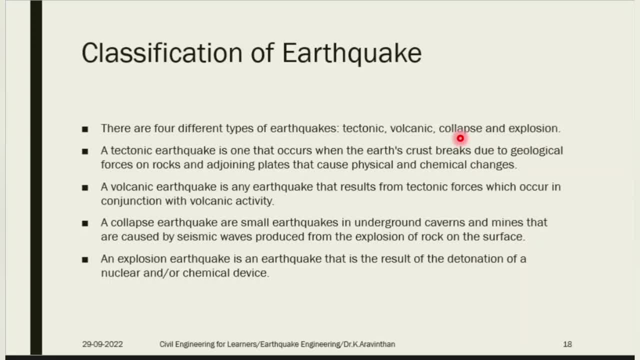 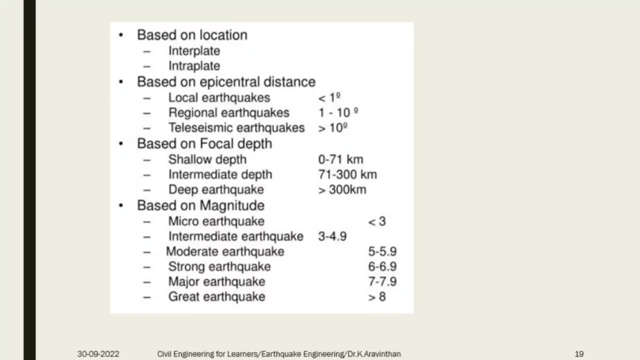 And mining is for manmade purpose, Explosion will also be there due to any war field. Nuclear explosion might be there. So due to that explosion, What happens? The earthquake might occur. There are further classification of earthquake Based on location. One is inter plate and another one is intra plate. 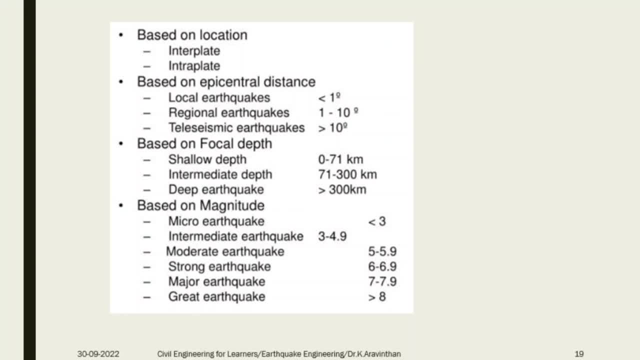 When the earthquake is occurring between the joint of the fault, Then it is called inter plate earthquake And intra plate earthquake is in between fault. Next one based on epicentral distance: If it is Below 100 km, Then it is local earthquake. 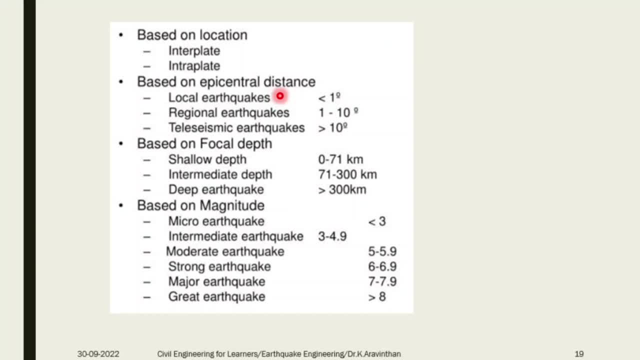 And if the earthquake occurs between 100 to 1000 km, Then it is called regional earthquake And tele seismic earthquake are greater than 1000 km. Based on focal depth, You can see 0 to 71 km And intermediate depth is 71 to 300 km. 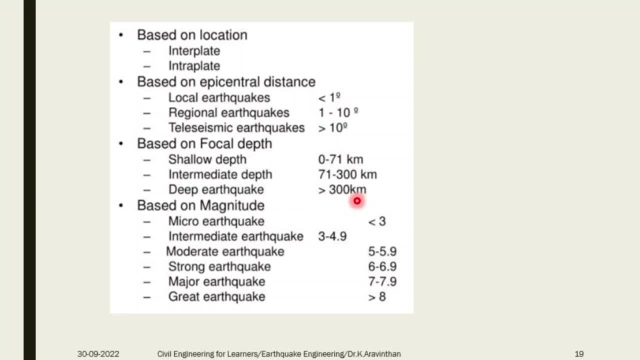 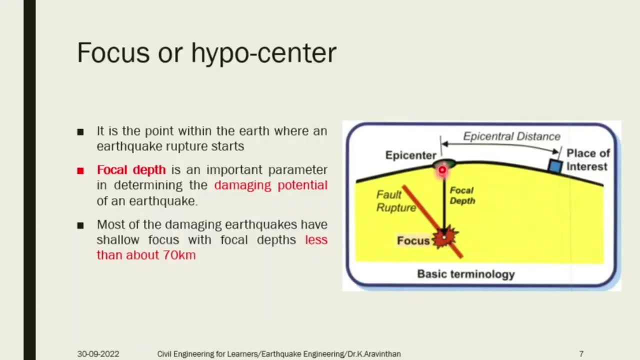 Deeper earthquake is greater than 300 km. So there is a difference between focal depth and epicentral- This is focal depth And epicentral- This is epicentral distance. This is the two difference If the earthquake is occurring below the ground. 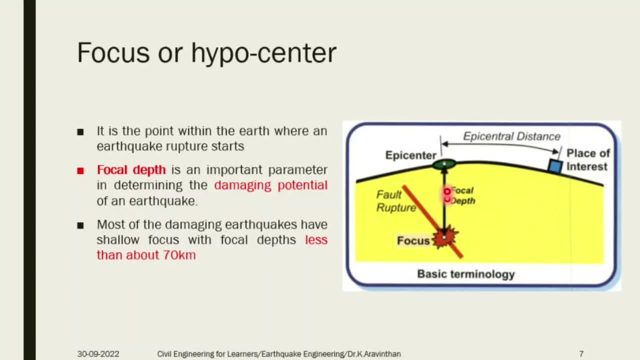 And this is the focal depth. So according to the depth, It is been considered as some earthquake. What do you mean by epicentral distance is, If it can cross more than 1000 km In distance, Then it is called epicentral. 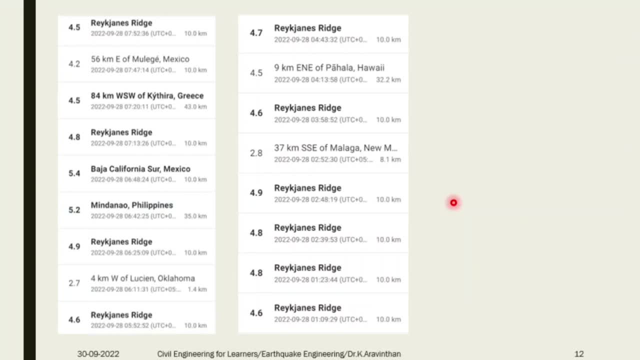 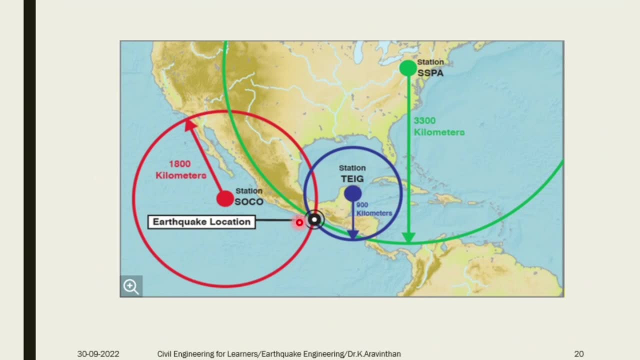 Focal depth. You can understand based on these types. Yes, By this example you can understand See some earthquake location. So if it is a station, The station indicates a seismometric station. If the seismometer is installed here. 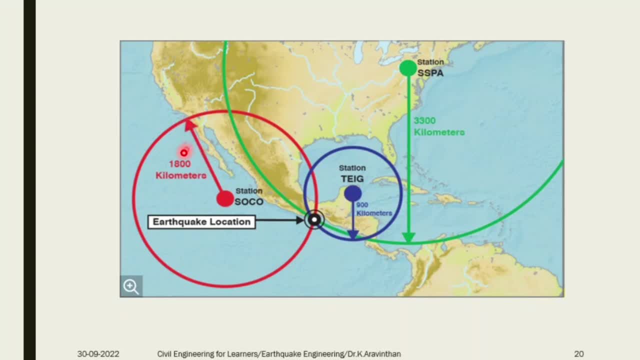 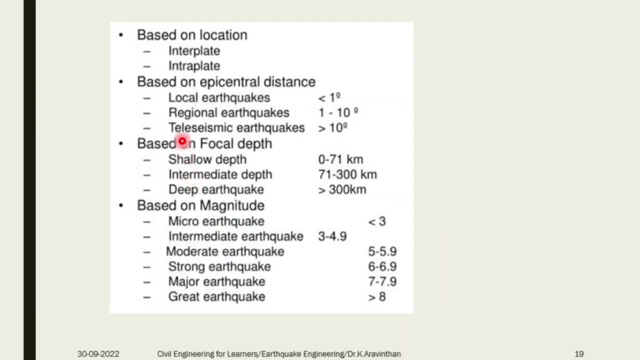 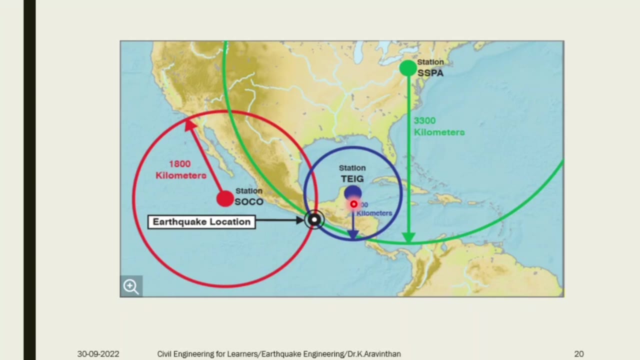 And an earthquake is being observed Till 1800 km, Then it is called tele seismic earthquake. So according to this case You can see Tele seismic earthquakes are greater than 1000 km. And If you are having another station here, 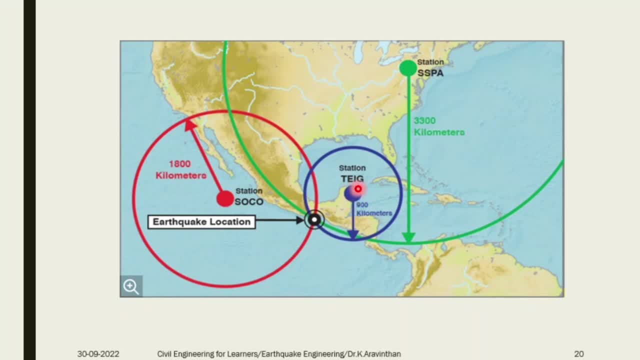 TEIG. These are all seismic station And they will record all the earthquake motions, Analyze, Monitor And develop the statistics. How to locate an earthquake? You can see Three number of instruments are being installed. All the three instruments will measure the same earthquake. 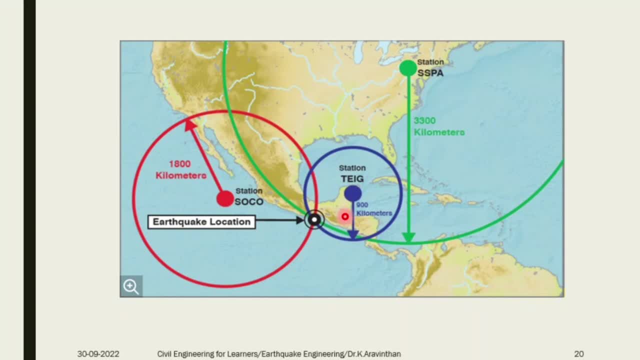 Nobody can physically go and visit the focal depth Where the earthquake is occurred. We cannot physically view it And even though it is below the earth, How we can understand their terminology and characteristic is By installing these instruments. One instrument will say that. 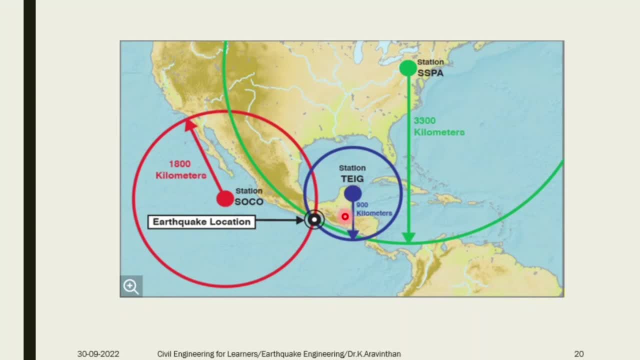 The earthquake occurred at 1800 km distance And this instrument identifies that An earthquake occurred at 900 km distance. And third one. So by this three number of Minimum, three number of instruments, You can able to locate. So at what time? 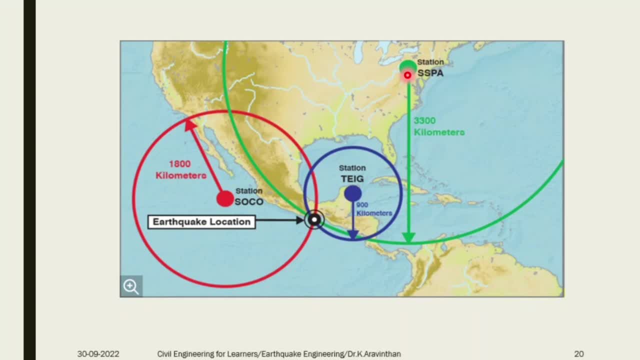 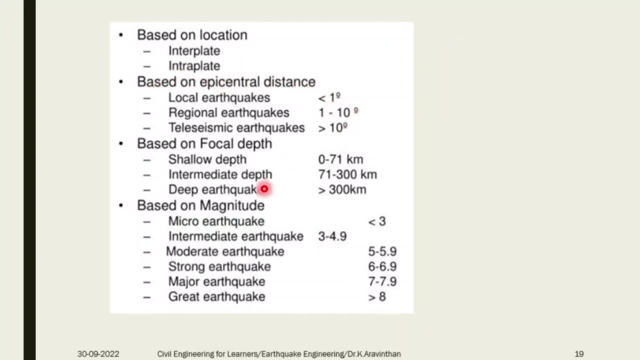 It would have started. It reached the station point. So, based on epicentral, Is what we have understood currently. Based on focal depth, How much depth The earthquake occurred? Is based on these three. Based on magnitude, You have micro earthquake. 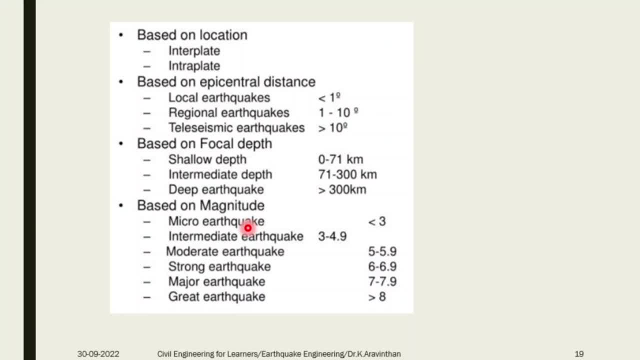 Dogs. They can sense. And intermediate earthquake is around 3 to 4.9.. This can be observed Slightly In the building And by the human. Moderate earthquakes are 5 to 5.9.. Strong earthquake 6 to 6.9.. 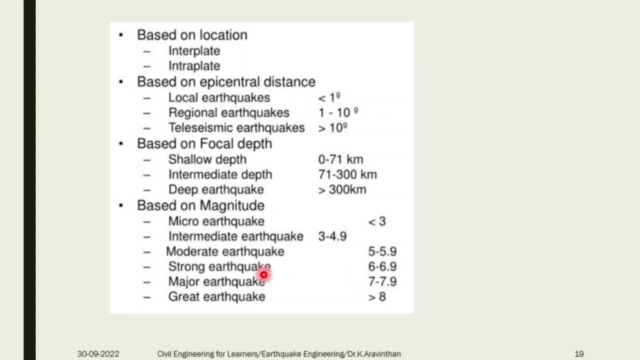 This strong earthquake Makes the property damage And, above that, If the earthquake is occurring, It does not make much property damage And life loss From the strong earthquake. We are very much interested. So how to tackle this strong earthquake? Around 180 number of earthquake. 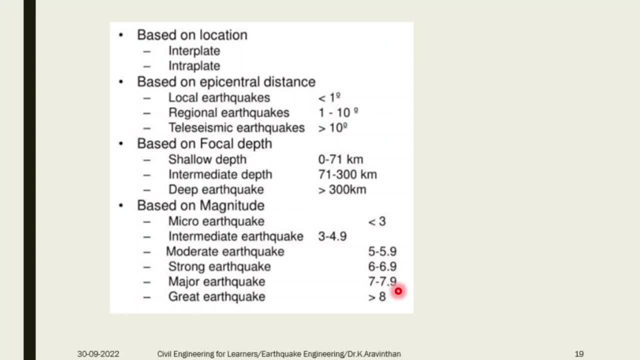 Is occurring throughout the world Continuously, year by year, But we are still suffering due to that Major earthquake- 7 to 7.9.. And finally, Great earthquake. What do you mean by great earthquake is If it is more than Richter. 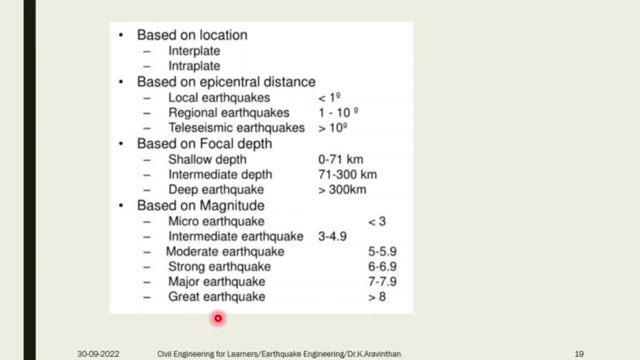 Scale of 8. It is called great earthquake, Where The majority of the structure gets collapsed. And if we are preparing for great earthquake, There is Too much of amount has to be spent To make the construction In India, Bhuj. 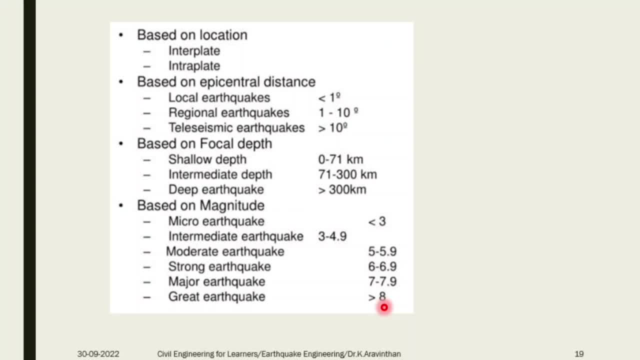 The state of Gujarat. You have a hospital Which is being constructed By elastomeric bearing. The total hospital is Completely covered with bearings. There will be a set of rubber pads And They are known as elastomers. So these elastomers- 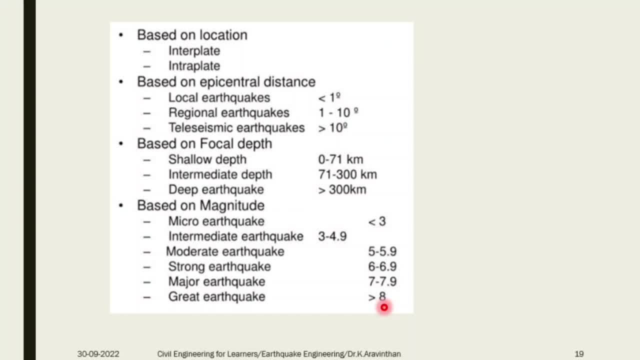 What will happen? They will be like a sandwich. The whole column Will be not connected to the earth. There will be a sandwich layer. And during an earthquake, What happens? This layer Tries to deflect In whatever mode The earthquake is occurring. 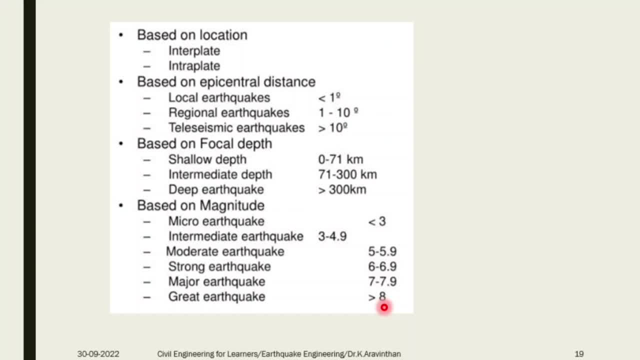 And The hospital can withstand Up to Richter 8.. That is The great earthquake During any cause In future. After the Bhuj earthquake Happened, The government Take an initiation Safety Against the Earthquake. 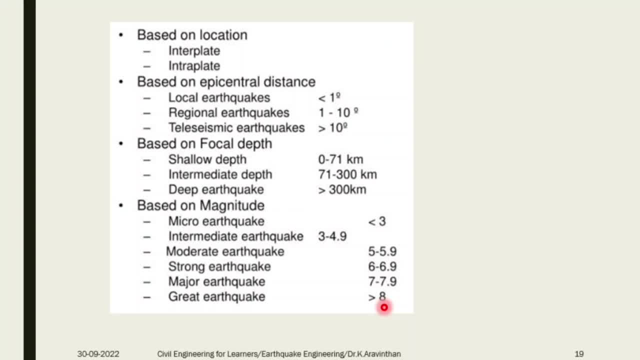 So, soon after The earthquake, You need The hospitals In order to run Successfully, In order to Cure the Patient During the Devastating earthquake. So at least In a state, There should be a Single construction. 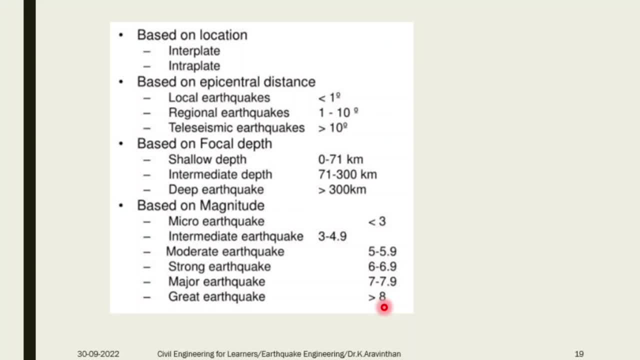 Like this, Whatever Might be The earthquake Structure, Like Hospital, Telecommunication Center And Monuments, We should Take care About All The Structures If, When You Are Speaking, 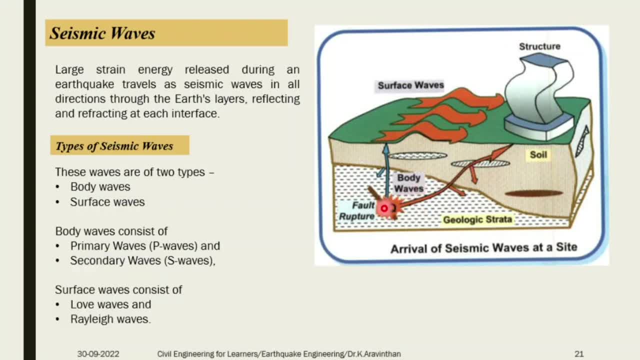 About Monuments. It Only Speaks About Civil Engineer. So Civil Engineer And The Structure. There Are Two Types Of Waves. One Is Body Wave And 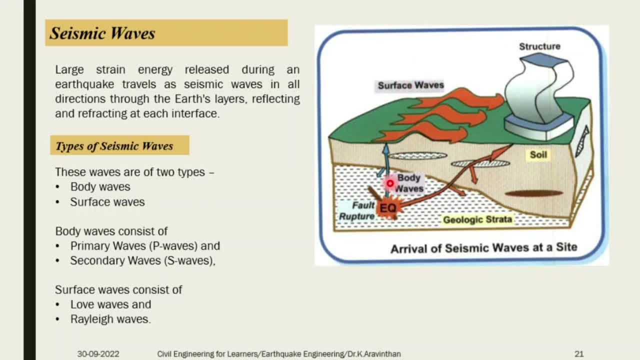 Another One Is Surface Wave. You Can Understand This Is The Earth Crust And This, If You Are Digging Deep, You Can See A Confined 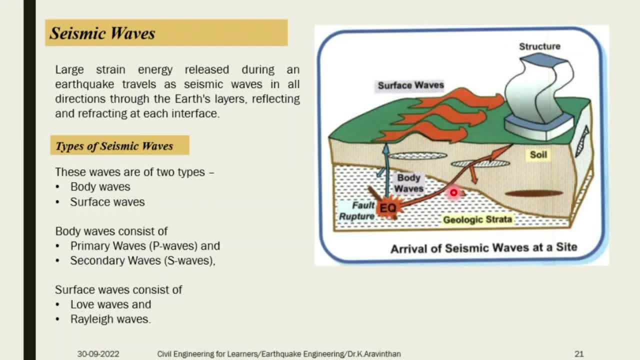 Aquifer Might Be There And There Might Be Some Different Types Of Soil In Between Certain Area, So When A Wave Travels As Seismic, 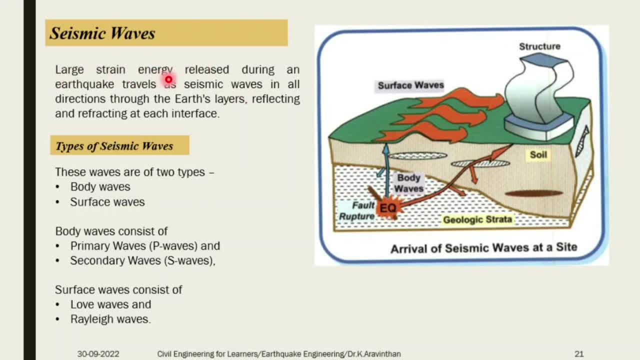 Wave. What Are These Waves? These Waves Are Strain Energy Which Is Being Released. When You Clap Your Hands, You Can Observe Some Vibrations. 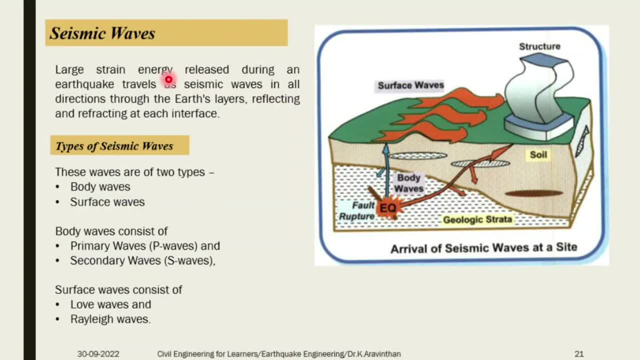 Fault Zones. So When It Strikes Or Fault Or It Can Dip, What Happens? These Wave Are Called Strain Energy. It Has Been Released, Transferred. 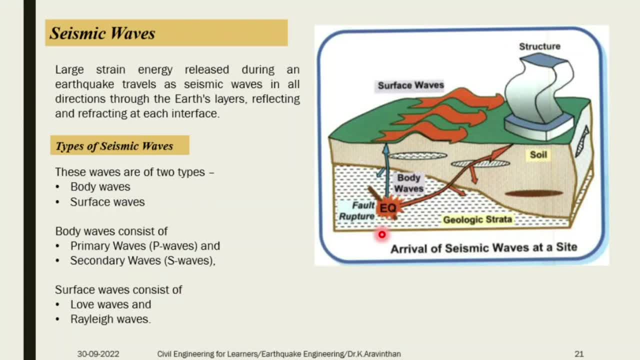 This Is Called A Core Mantle. And Then You Have The Crust, The Waves Which Go Into The Earth Is Not Going To Get Damage. 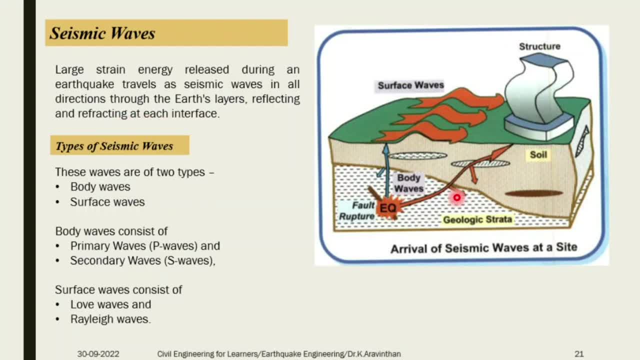 For Any People. So We Are Not Interested Similarly In A Pressure Cooker. What Happens? Slowly The Heat Gets Increased. So If It Is, 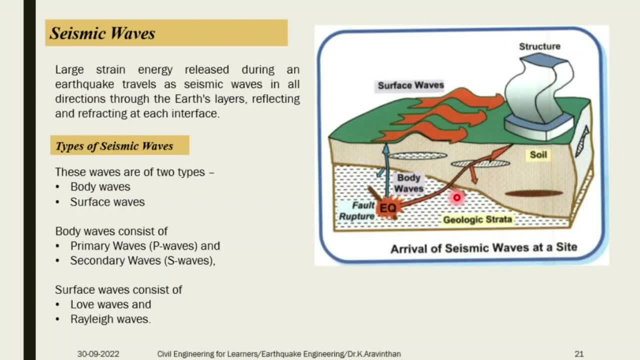 Getting Increased, The Pressure Has To Release Somewhere Or The Other They Have. These Are The Places Pressure Releasing Points Are Called Volcanoes Active. 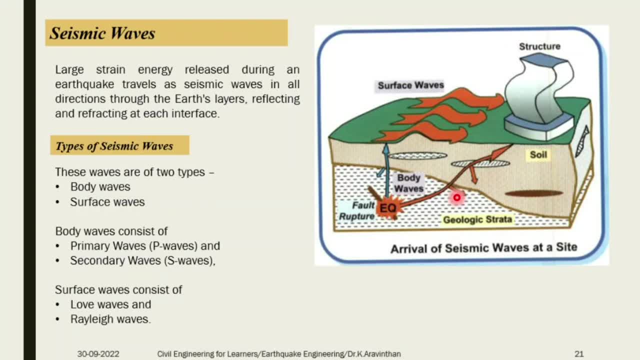 Volcanoes. So They Have The Knob In Order To Release The Energy. So What Are The Energies? There Are All Nitrogen, So These 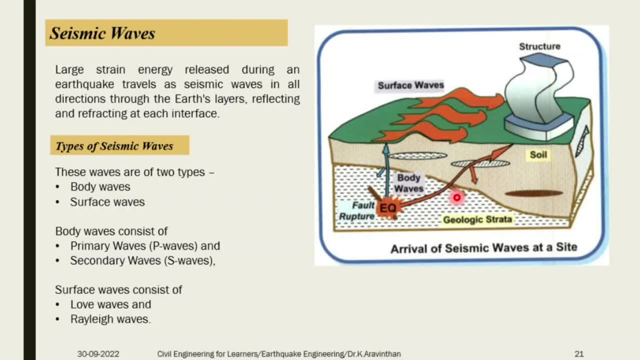 Are The Essential ingredient In The Environment, Because All Of The Nutrients We Have A Use To Prevent A Fuji From The Planet, Or are called surface waves. Body waves are consist of two types. one is primary wave. 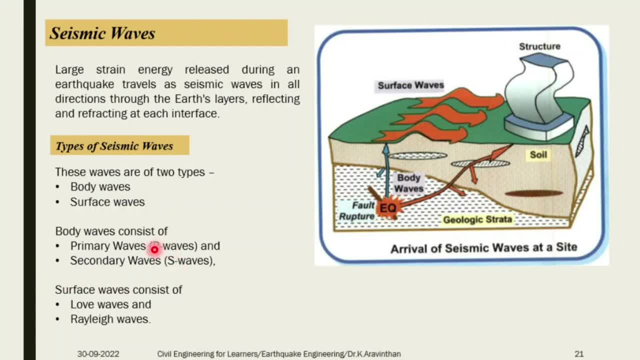 and another one is secondary wave. It might be called P wave and S wave. in short, Surface wave consists of Love wave and Rayleigh wave, Professor Love, who identified the different character of the wave, and next thing is Rayleigh wave. He is professor Rayleigh and he identified certain characteristics in a 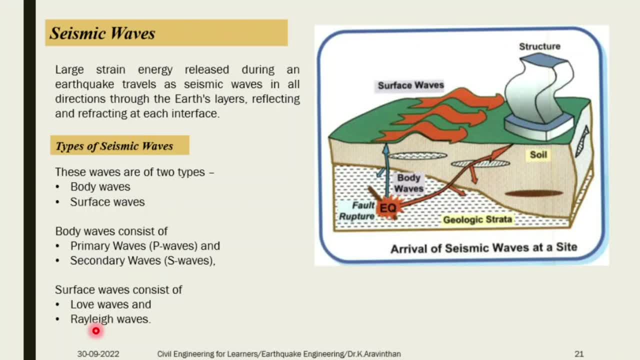 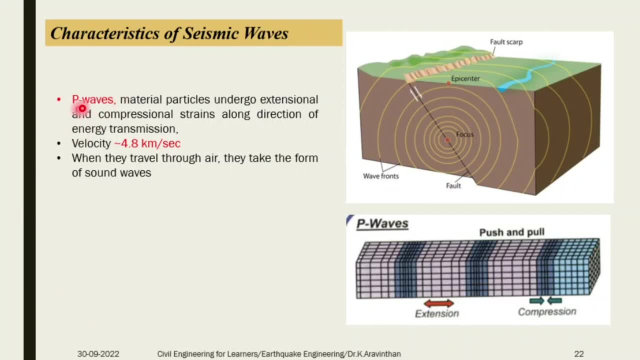 earthquake, So it is generally called as Rayleigh wave. Okay, when we are understanding characteristic of wave, first wave is called P wave. What I mean by that is primarily, you can understand fault number one, fault number two: It is getting sheared. and if it is sheared, what happens? from the focus, the 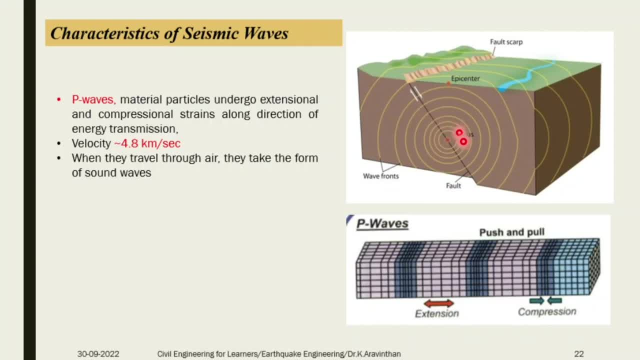 earthquake is getting generated and it is being transferred in all the directions. So when it has been transferred, you can see this fault area. This is the fault area and this is the focus. When the wave is traveling, it will travel in form of push and pull. So from the starting of the focus, it waves, it transfers in this manner. 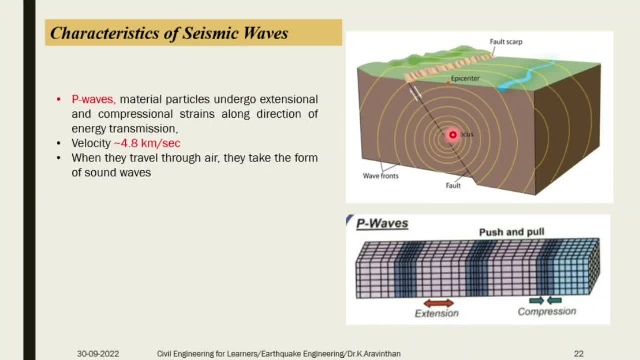 So it is the fastest wave in the four waves. Primary waves are the fastest wave When an earthquake is going to occur. if you are in a building, if your building is pushing and pulling, then you should understand that there is a severity and there is an earthquake is going to get happen. 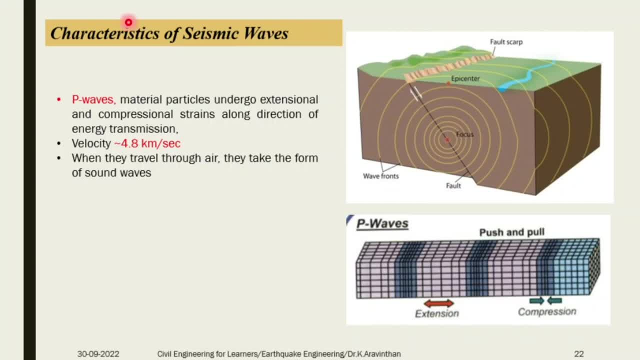 Soon, you have to act accordingly. And it travels at a speed of 4.8 km per second. So it is unimaginable. and it is more than severe Sound, So it travels more quickly than sound. When they travel through air they take the form of sound waves. The particle generally goes under extensional and compressional strains, So it extends and compresses. So this is the character of P wave. 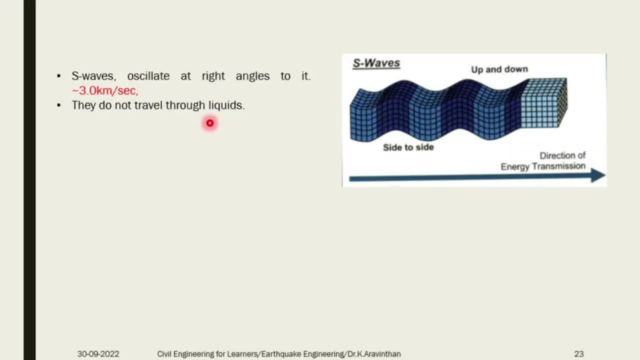 The next wave is called S wave. S wave is generally a wave which is moving up and down. Its velocity is less than P wave, So S wave has a velocity of around 3 km per second. They do not travel through liquids. So if there is any liquid part, if the wave is traveling and any confined aquifer is there, what happens? 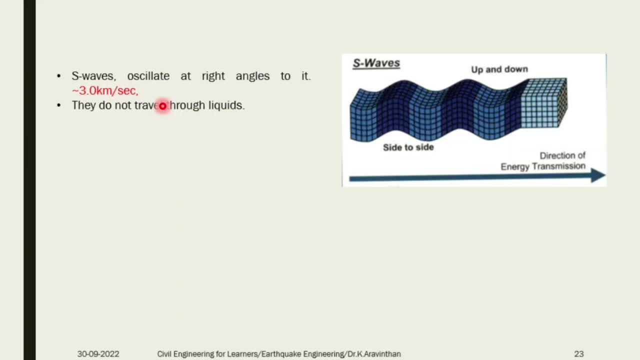 It travels through the confined aquifer. It travels in up and down mode. When it matches the confined aquifer the liquid collapses, the wave, and after the aquifer it cannot pass through. So certain waves are sent back. This is the direction of transmission. S wave goes through up and down motion. 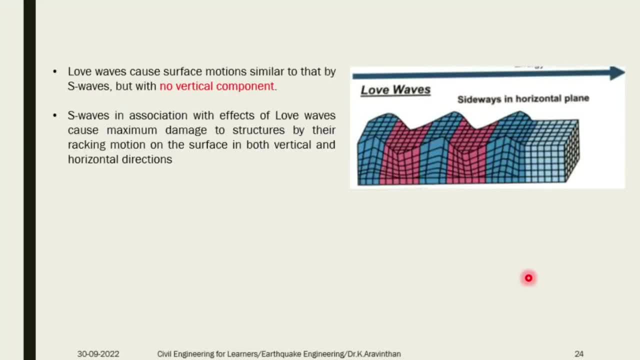 Third type wave is called low wave, Then a horizontal wave. Primary wave is pushing and pulling, So it is compression and tension. So secondary wave is going up and down, So the wave will go up and down. So the low wave goes in horizontal direction. If the wave is going in horizontal. 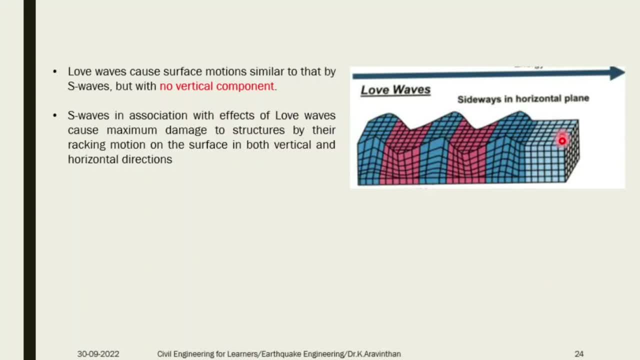 It is called zig-zag mode, that is, in sideways. This is the best example. If the wave is going in sideways, then it is called low wave. It does not have vertical component, It only has horizontal component and S wave associated with low wave causes maximum damage.